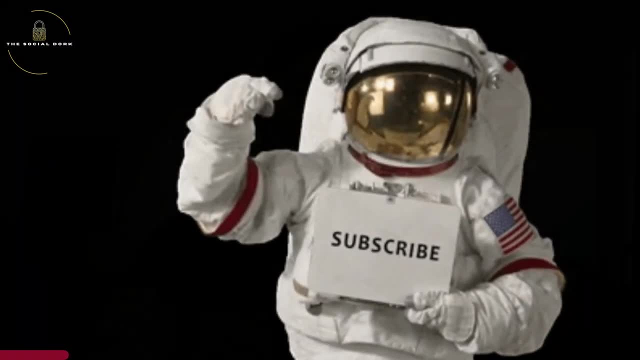 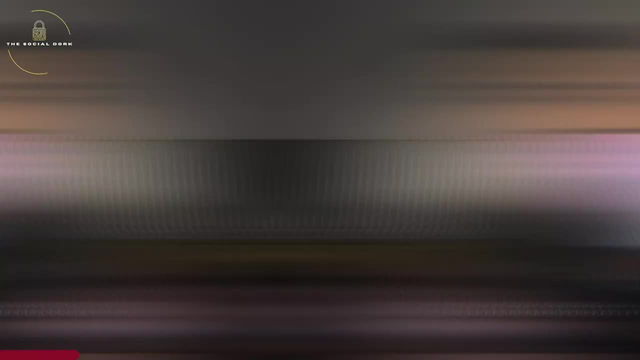 subscriber. do show some love. hit the subscribe button and the like button on this video. In this video I'm going to speak about the help desk. Being a help desk engineer has numerous benefits, and the help desk in itself is also considered to be the holy ground, or? 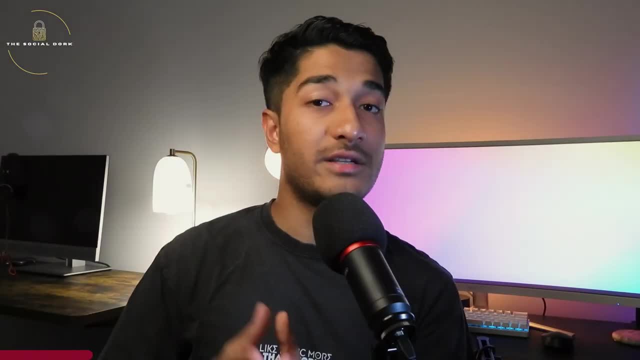 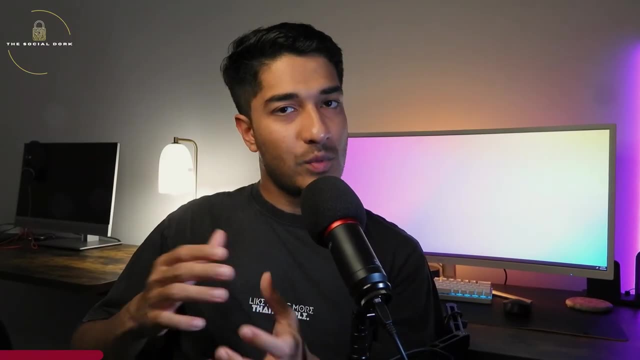 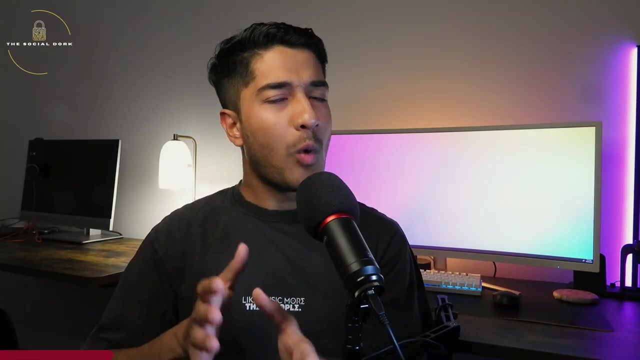 the best starting point if you want to achieve great things in your tech career. Why exactly am I biased towards help desk engineers or a help desk position? Reason being: that is where exactly I started my career as well, and I saw numerous benefits of working as a help desk engineer. Therefore, in my one year of working in that field, I came up with 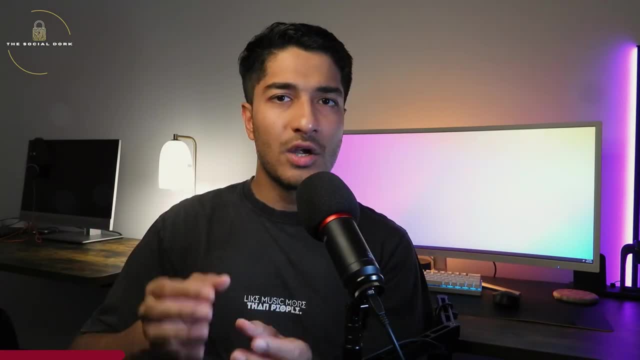 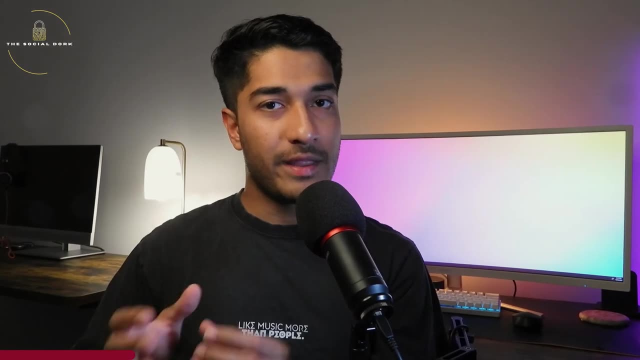 five points that I can use to potentially convince you guys why this decision could change your life. The number one advantage of working in the help desk is that it's easy to get a help desk position. The number one advantage of working in the help desk is that it's easy to get a help desk position. 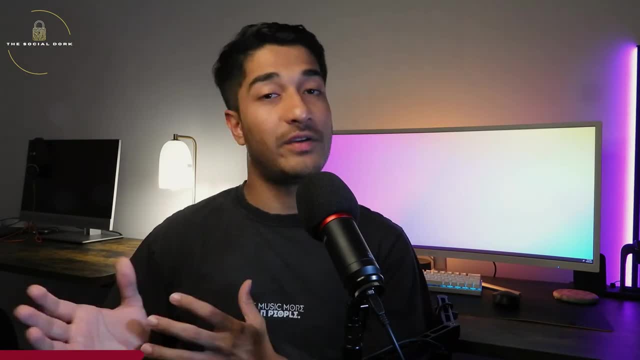 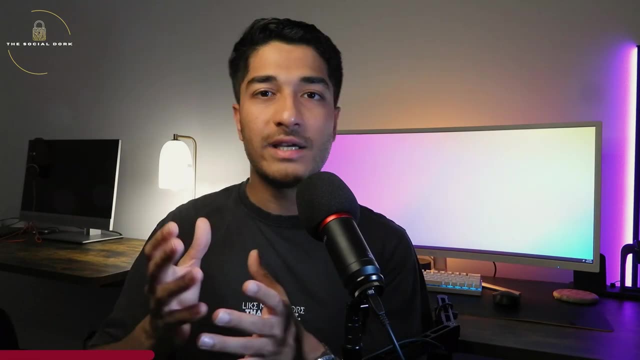 What exactly I mean by this is when you're looking for, let's say, for example, junior network engineer, junior security analyst or junior cyber security roles as your first ever entry into the industry, it's possible that that job hunt might be a little challenging A lot of companies out there. sometimes have unrealistic expectations where they want candidates to have certain years of experience, even for a junior role. Look, I've been there so I know it's not possible at all. Help desk roles, on the other hand, are more open to higher hiring junior level candidates. As a result of this, it makes your entry into the industry. 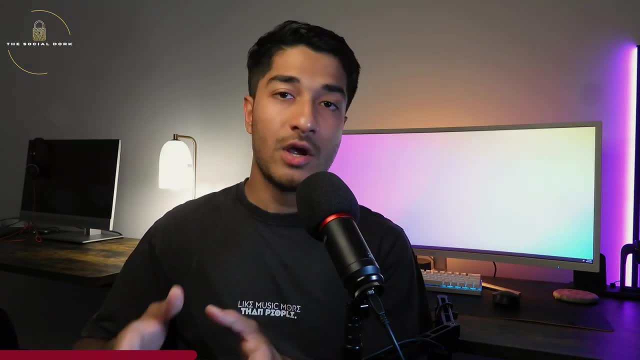 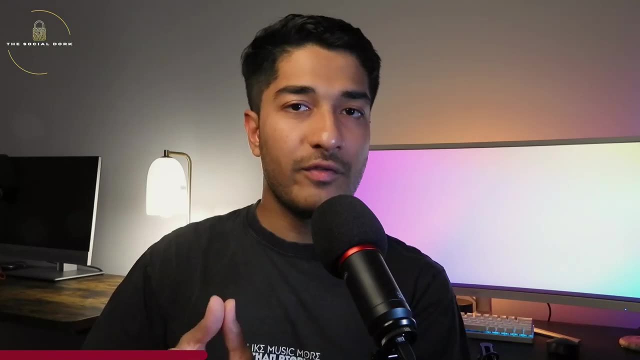 very easy and look. it's all about getting into the industry. Once you get in, you can work in the help desk for a year, year and a half, and you can then branch out into more specialized fields. Therefore, whenever I speak to any budding engineers, I always emphasize on 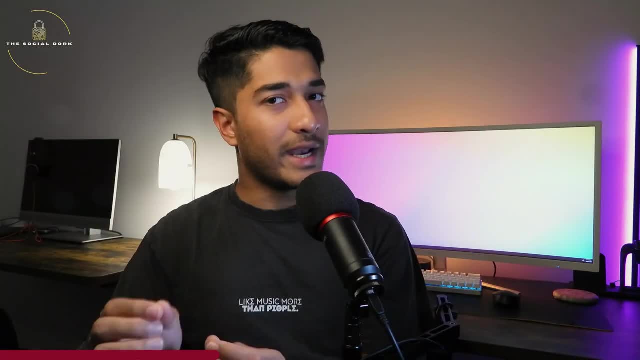 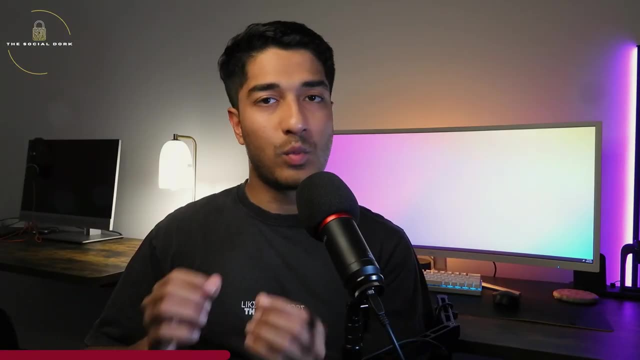 the importance of applying to help desk roles as well, because it's all about getting in. Once you get in and you cement your position, you can then climb the ladder. and this brings me to the second point, which is, once you get your help desk role, what that does is 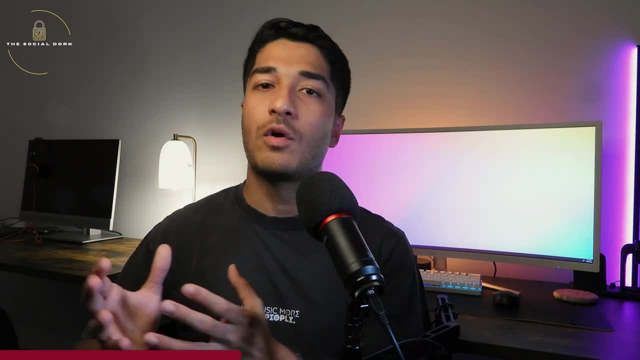 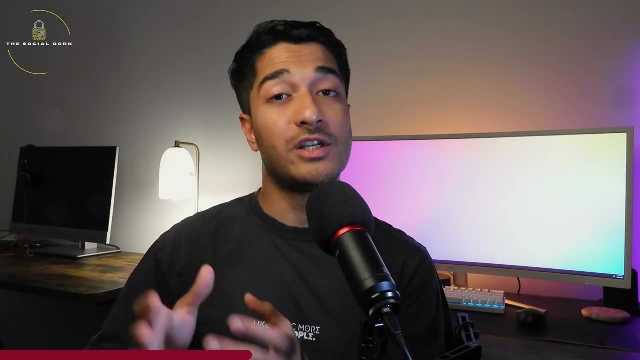 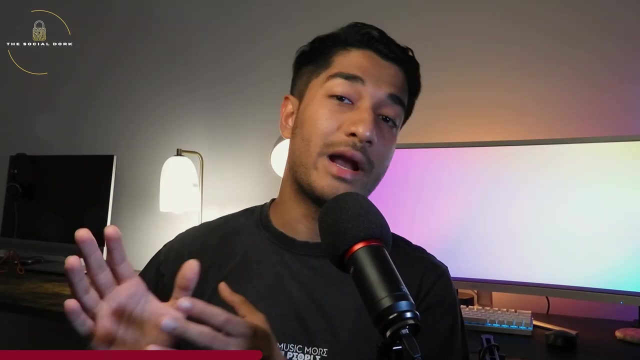 is, it helps you strengthen your foundational, core level concepts. I'll give you an example. when I was working as a help desk engineer, my role was mainly to configure digital displays, smart displays, which literally had nothing to do with netbook engineering or where I wanted to go. 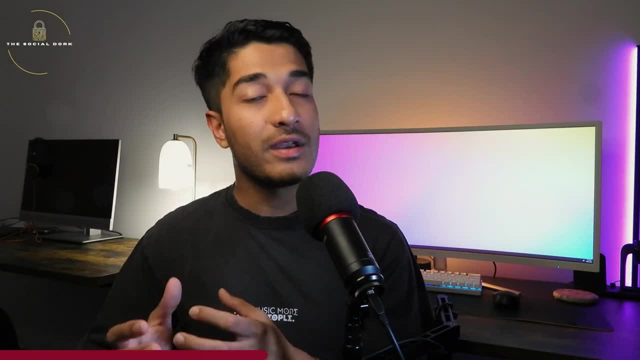 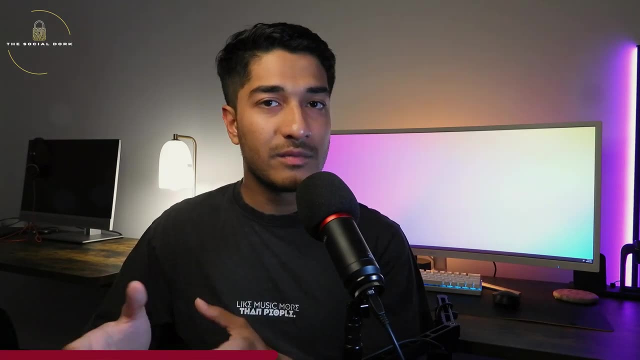 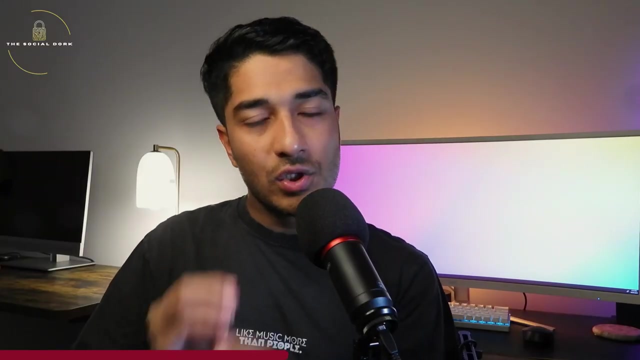 at the time. but what it did was it helped strengthen my foundational level concepts of working with systems, working with devices, working with the different types of operating systems, better understanding what networking of devices actually is. and look, strengthening your foundations is so, so important if you want to have a. 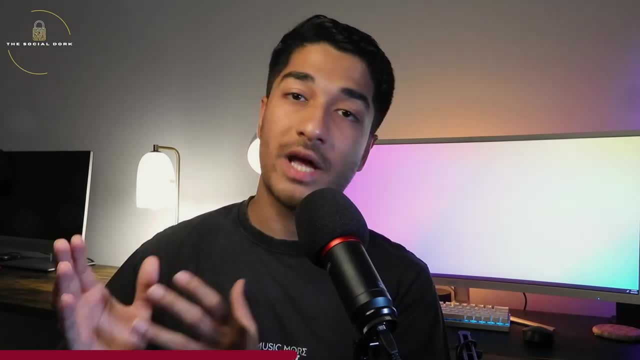 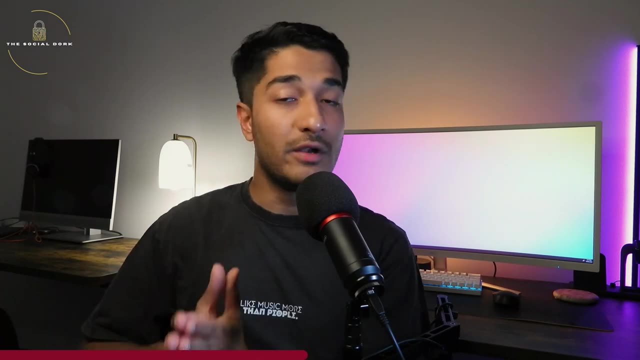 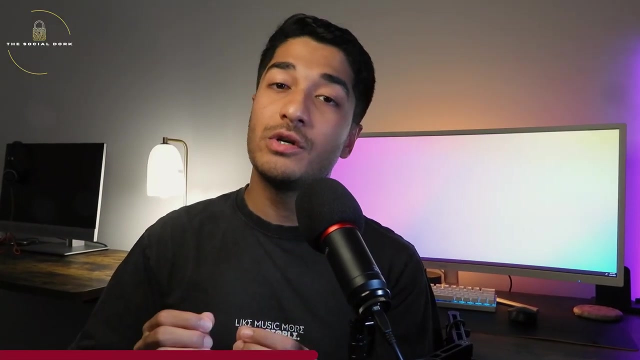 successful and long career in network engineering or cybersecurity. therefore, try to get your first help desk role and then also try and strengthen your foundational level knowledge and you're already setting up yourself to have a successful career. the third point is exposure to diverse technologies. working as a help desk engineer gives you the opportunity to work on pretty much every 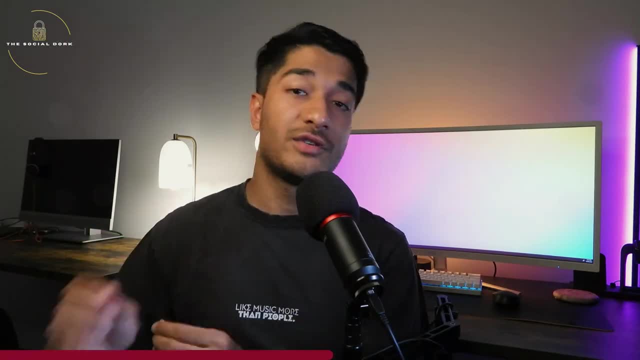 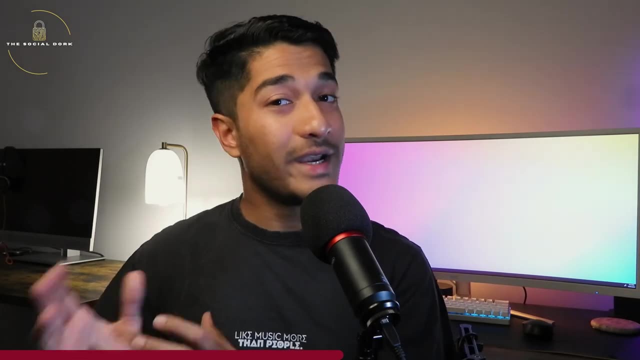 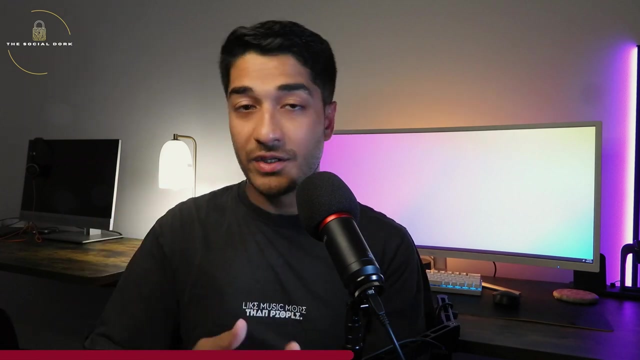 IT system that's part of your organization's IT infrastructure. you've got a troubleshoot and fix customer related issues around, let's say, multiple applications, operating systems, etc. so what this does is it gives you an insight into, let's say, working of applications, printers, networking, Wi-Fi. 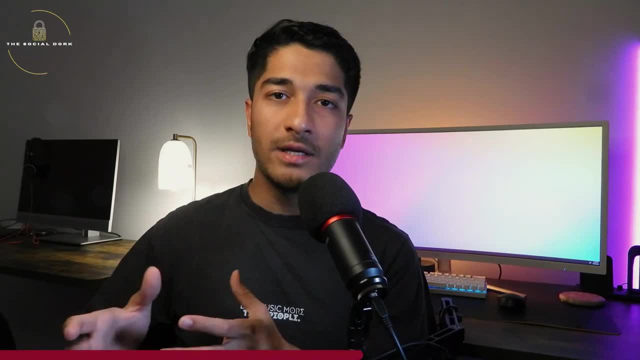 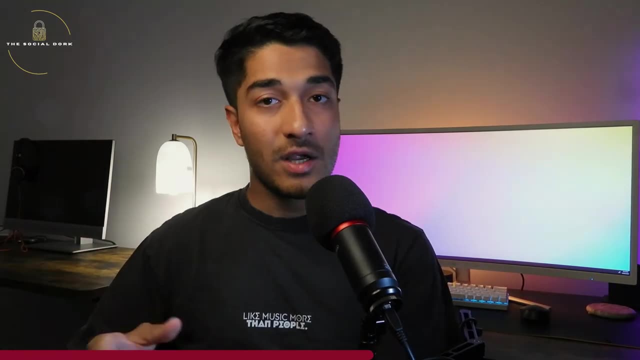 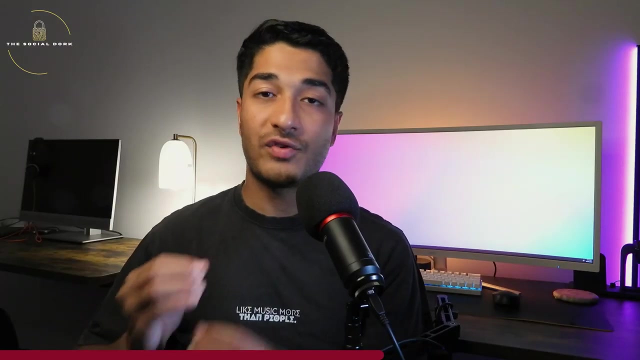 and so on. so, as you already see, if your goal is to be a network engineer, you're not just exposed to network engineering related things, but you're also then exposed to systems, software engineering applications, etc. the biggest advantage of this is that it strengthens your skill set. so when you're then applying 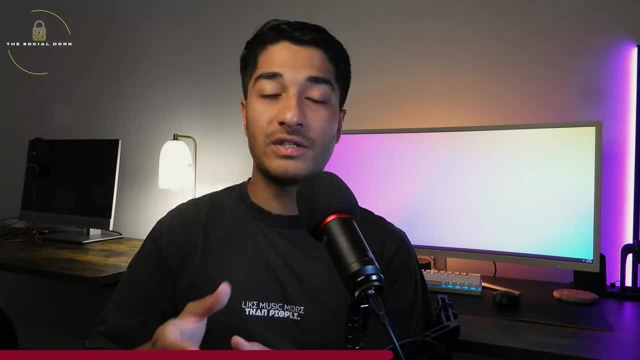 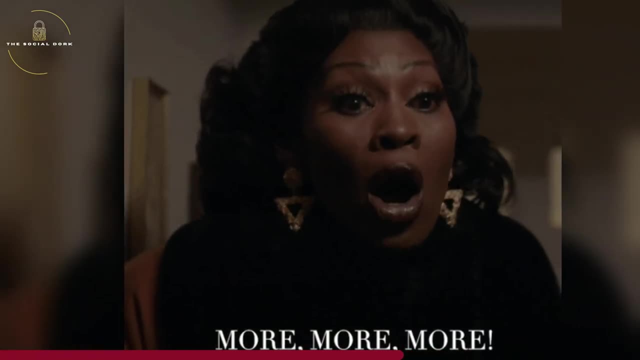 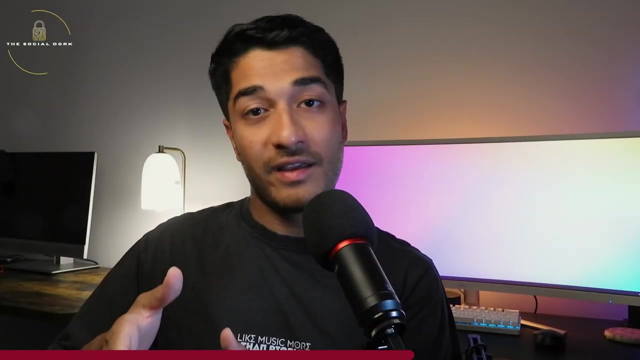 for your next role. you can boast about these different things you've worked on on your resume and when it comes to tech roles, the more the merrier because most organizations they prefer candidates that can do way more than just what the job description says they've got to do. therefore, your exposure. 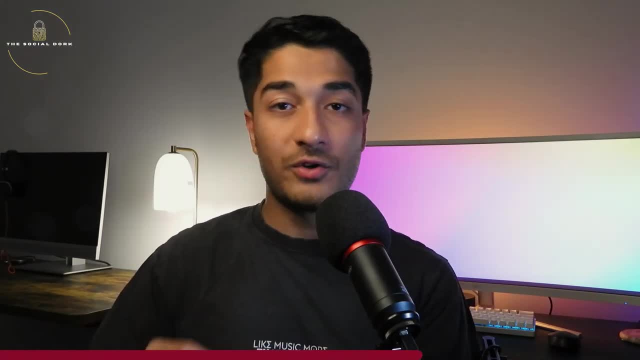 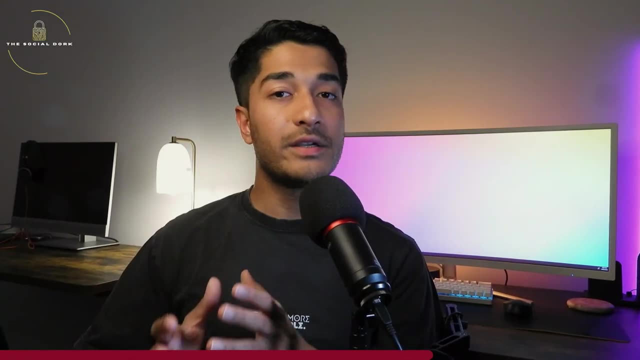 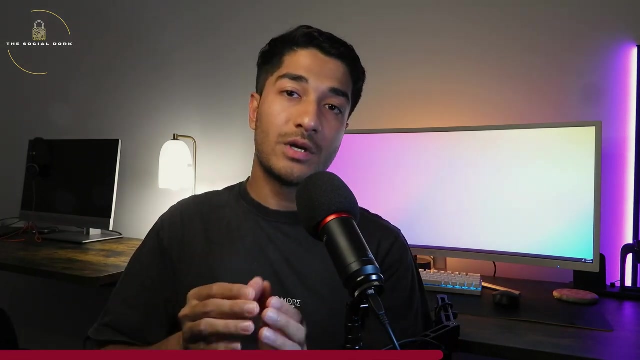 to these different technologies and working with different platforms already gives you a very big advantage over other candidates when you're looking for more specialized job roles. the fourth advantage of working as a help desk engineer is customer interaction. the primary role of a help desk engineer is to troubleshoot customer related issues. now, as I've already mentioned in the 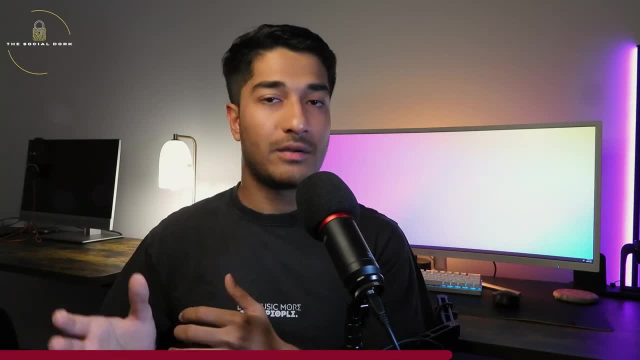 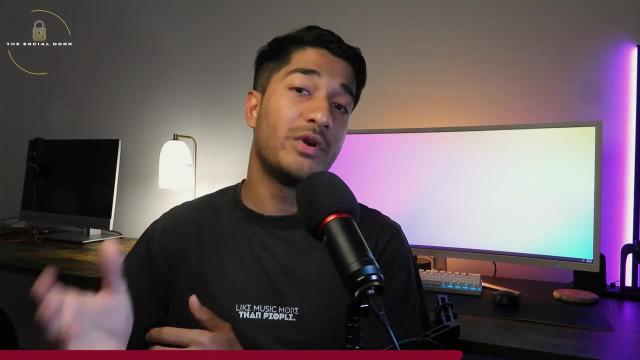 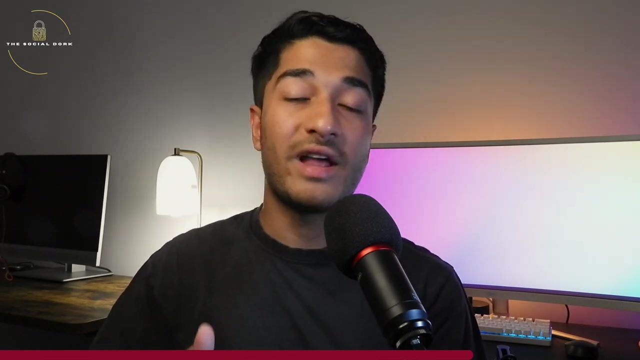 video. I've already spoken about this. it could be that you know a client or a user of your organization has issues with an application, or they are not able to log in, use the printer, etc. what this requires you to do is speak to them, understand their problem and then ultimately try and troubleshoot and fix. 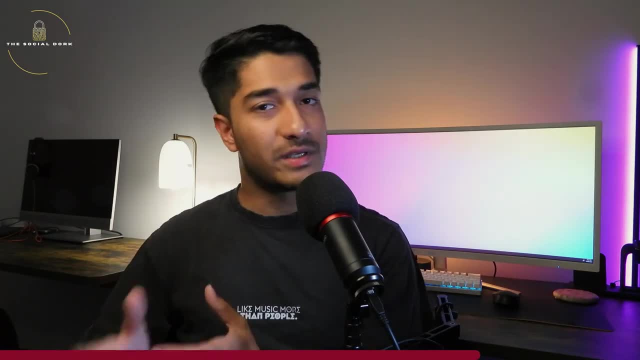 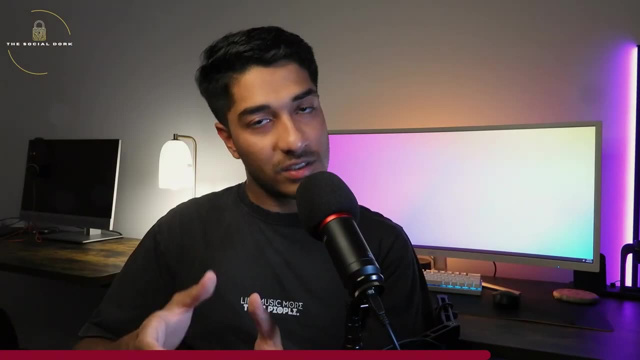 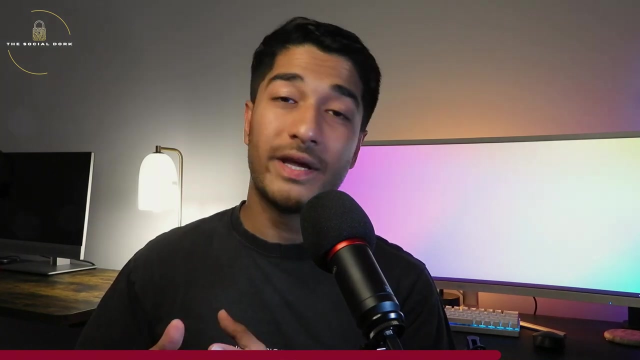 their issue. working in more specialized roles like network engineering or cyber security needs you to work with stakeholders, vendors, clients, etc. and having this customer interaction experience from the help desk can prove to be very valuable. and, look, I can't stress enough how working with difficult or impatient customers or 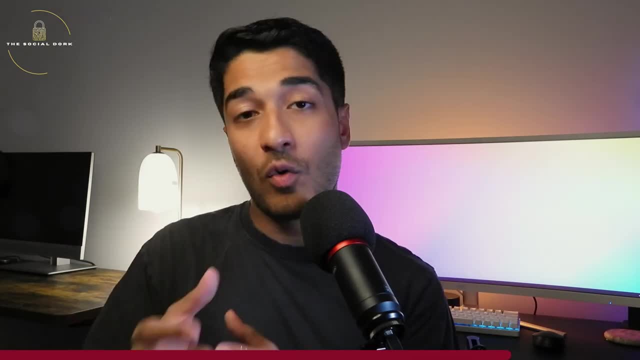 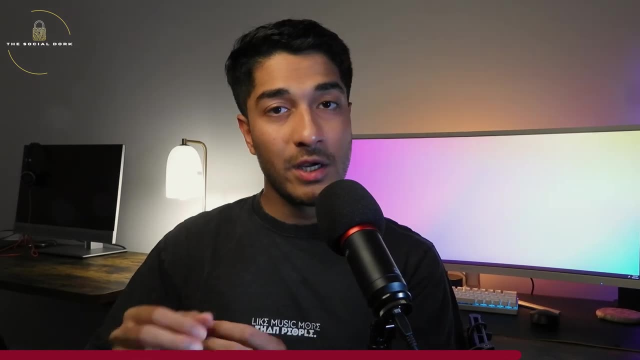 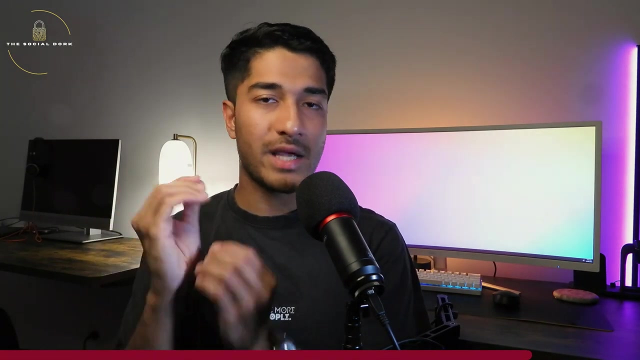 clients in a help desk role can add to your overall experience as a tech professional. and the fifth and final point is that the help desk will offer you opportunities to branch out into different IT specializations. now, when I started this video, I said that if your end goal is to be a cyber security or 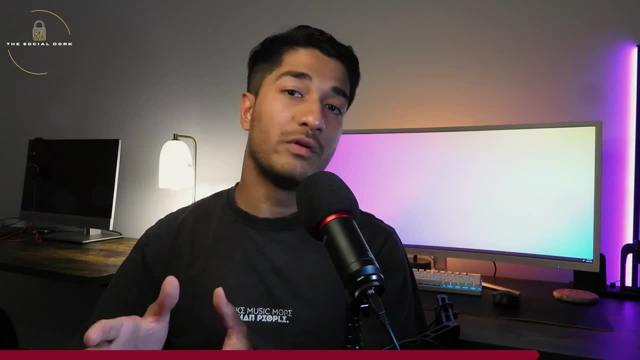 network engineer, then you should be able to work with a lot of different IT professionals and helpdesk is the perfect beginner role for you. but let's say you're working in a help desk role for a year or a year and a half and you're then exposed to. 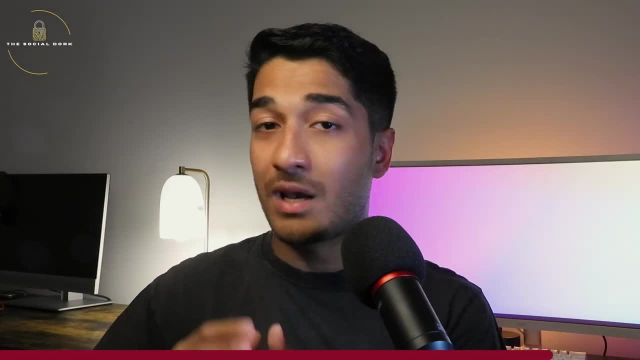 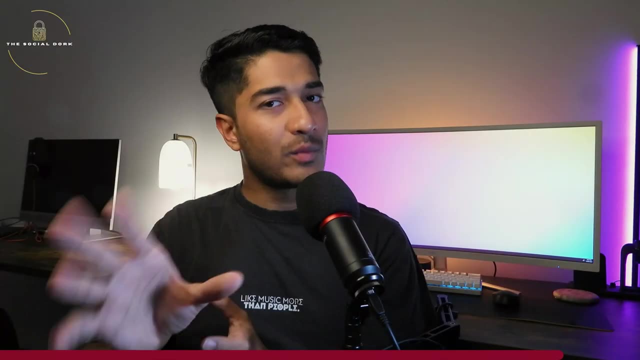 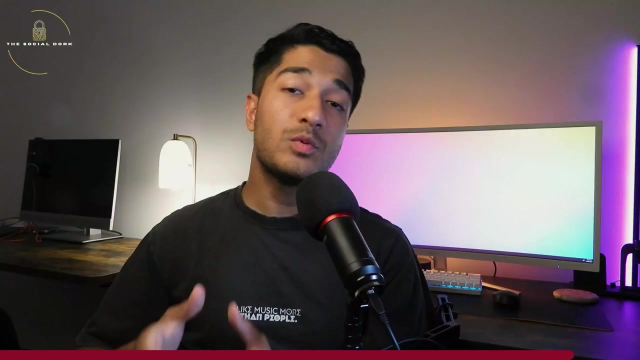 coding or system administration, cloud networking, etc. you can also then choose to branch out into these fields. therefore, not just network engineering or cyber security, but working as a help desk engineer can then open many doors for you to explore, and that's what working in information technology does. right, you've got these. 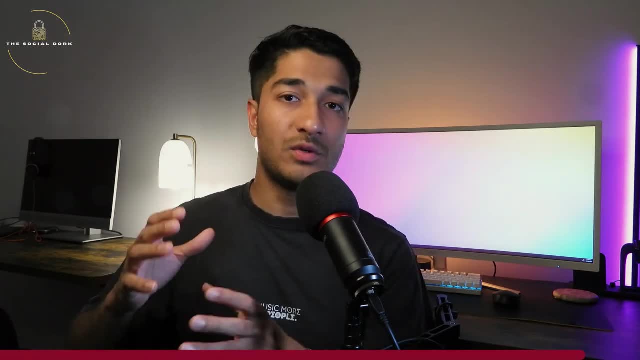 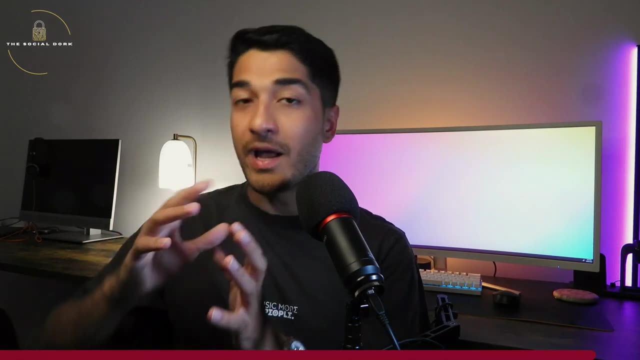 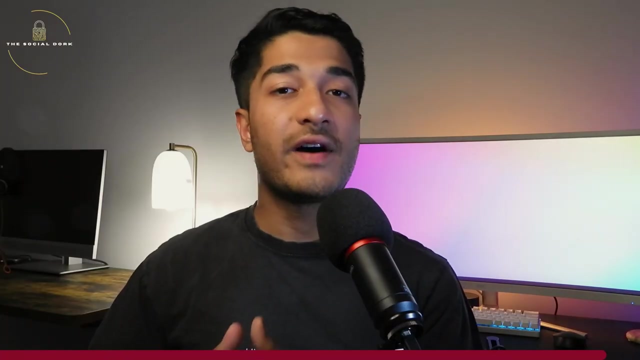 opportunities to further branch out into more specialized fields within IT and, as I said already, working in a help desk role and working on these diverse technologies gives you that opportunity and builds a solid foundation for you to do so. so there you go. these were the five reasons why working in a help desk. 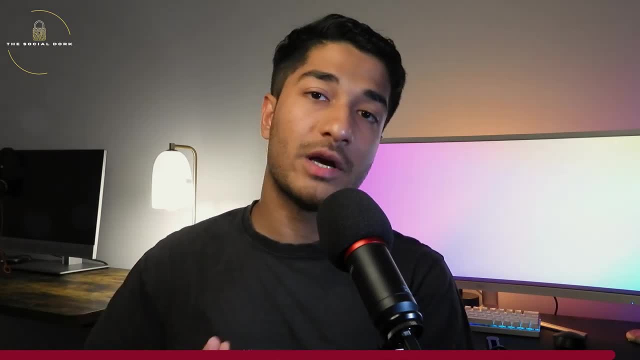 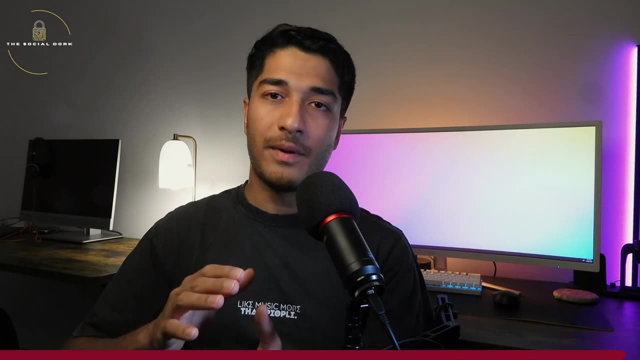 role can prove to be very crucial if you want to have a successful career in the networking or cybersecurity space. now look, there are many points that I could add to this list, so let's get started. but I didn't want this video to be very long, but if you feel that I've missed any, 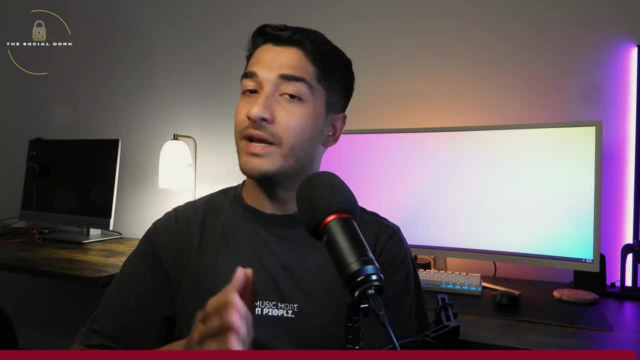 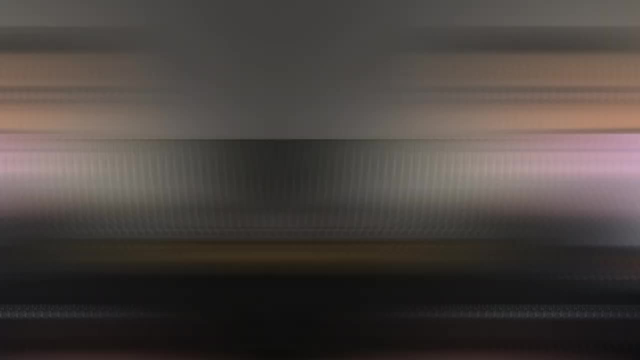 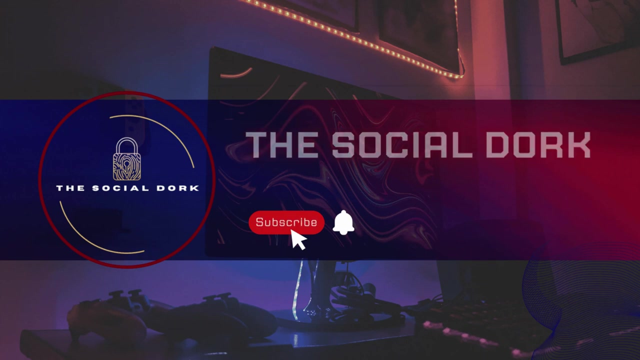 points out or you have a certain idea when it comes to help desk roles, please put it in the comment section. drop a like on this video, subscribe to the channel and I'll see you in the next video. thank you so much for watching and I'll see you in the next one. take care, and I'll see you in the next one. bye.